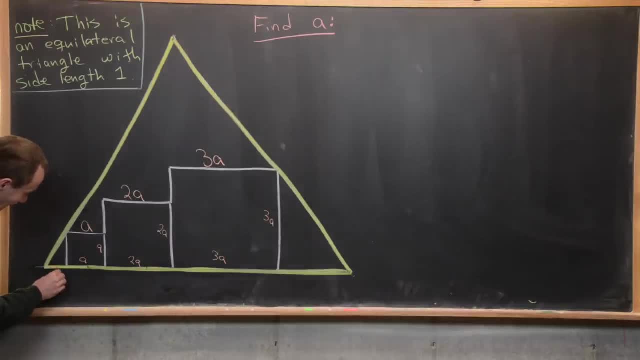 that if I set this length down here equal to x, then I have some sort of relationship between a and x, given that I know that this angle measure is 60 degrees, or pi over 3 radians. So let's recall up here that tangent of pi over. 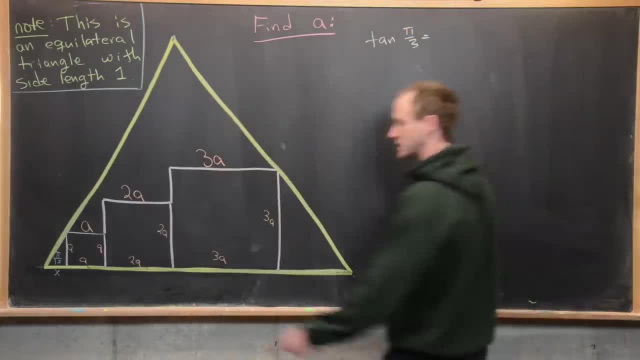 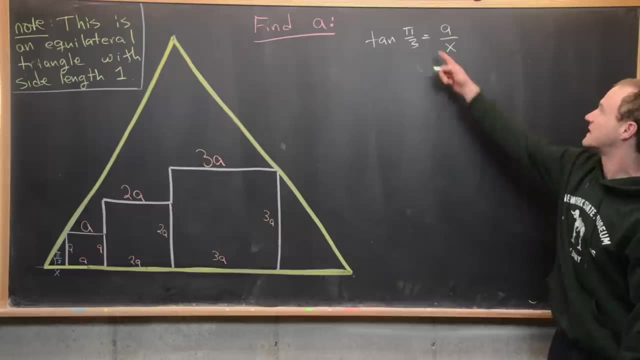 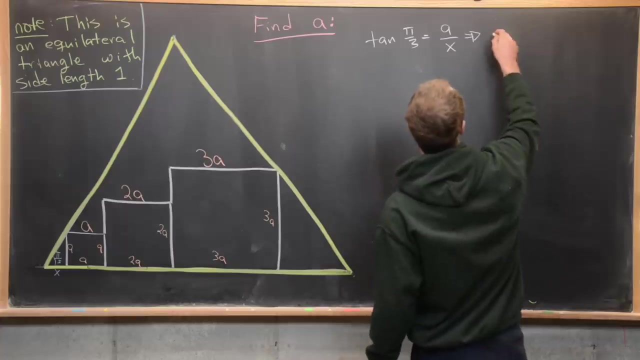 3. so that's going to be opposite over adjacent. so that's going to be a divided by x. Great, but we know that the tangent of pi over 3 is equal to the square root of 3, so that tells us that a equals the square root of 3x, or that x equals a. 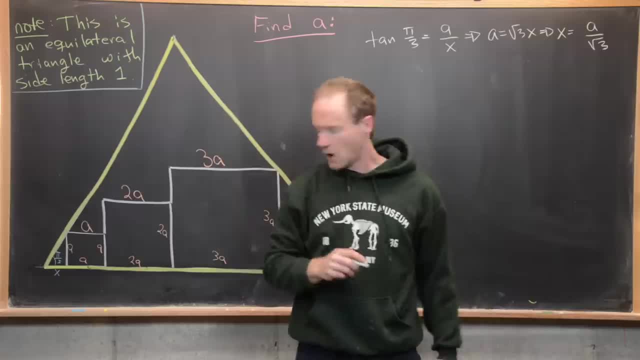 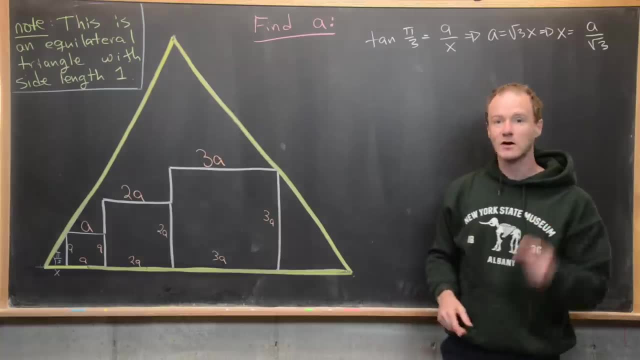 divided by the square root of 3.. Okay, so now we've got x in terms of everything, but what's the plus or minus factor for this? Well, let's first do the a, which is good to know, and then, furthermore, by the angle, angle, angle theorem, we know that this: 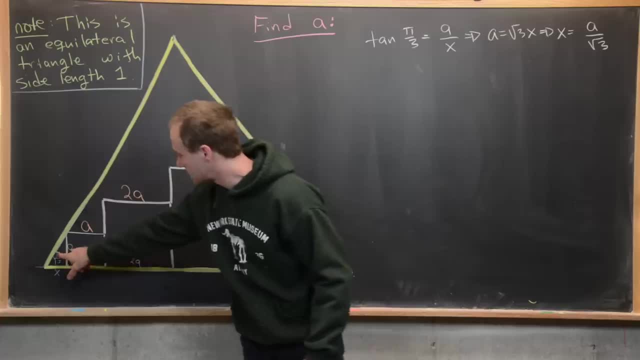 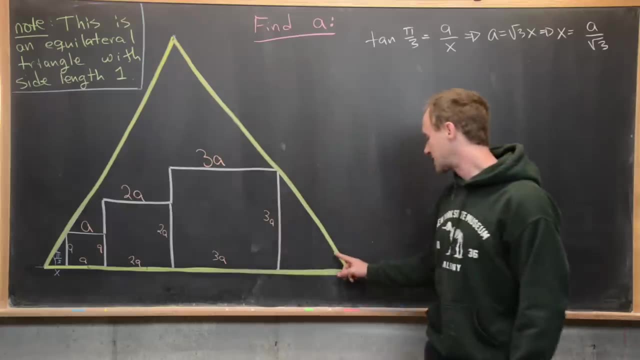 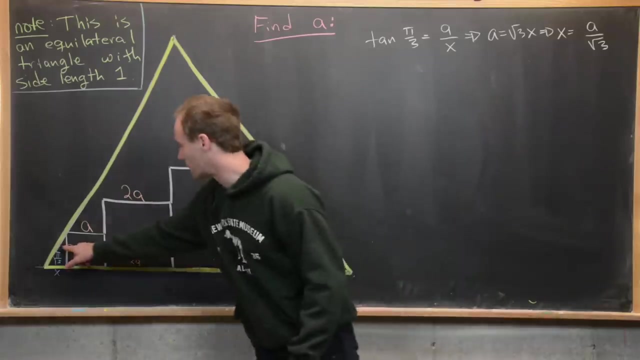 triangle over here and this little triangle over here are similar, so we know that they both have right angles here. and then next, we know that this is also going to be 60 degrees, or pi, over three radians, which means that this angle and this angle are the same, and so, like I said, by angle, angle, 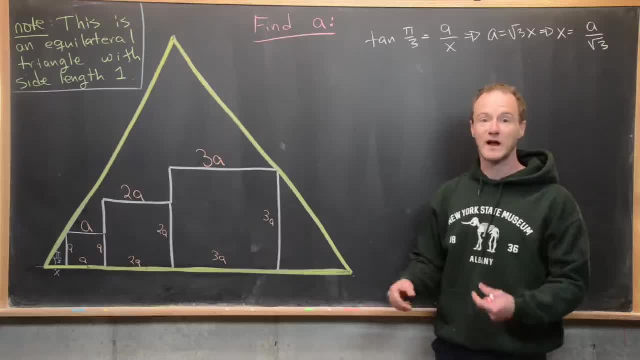 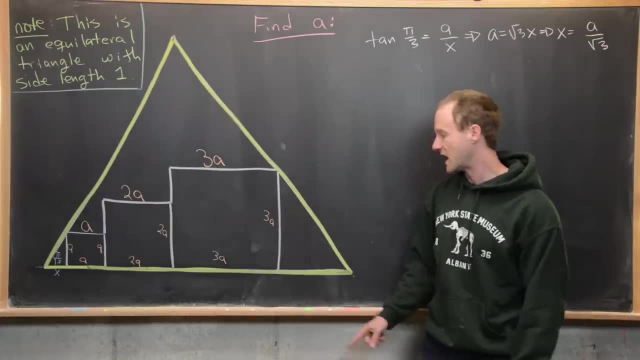 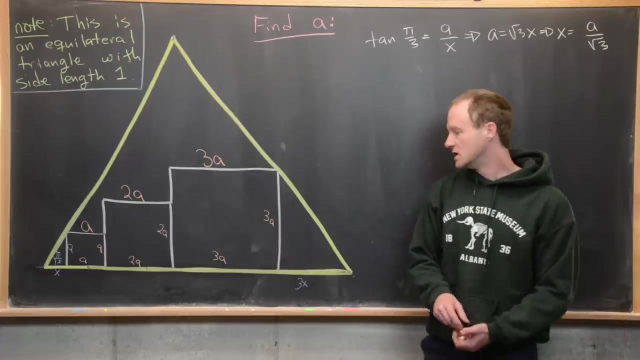 angle. these are similar triangles. that means the ratio of their sides are the same. so this side is three times the length of this side, 3a versus a. that means this down here has length 3x. good, so now let's put this together. we know the side length totally of the bottom will be equal to. 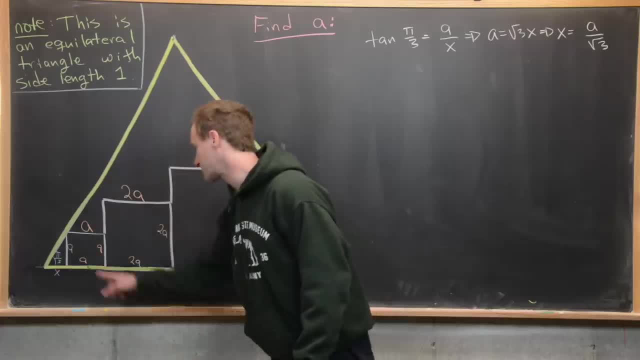 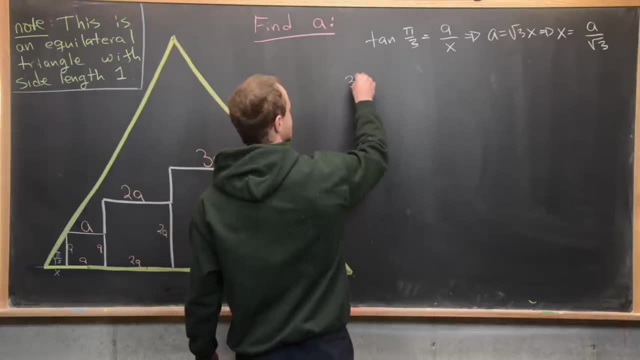 1, but that's also equal to 3x plus x plus a plus 2a plus 3a. so let's maybe also notice that we have 3x plus x plus a plus 2a plus 3a is equal to 1. 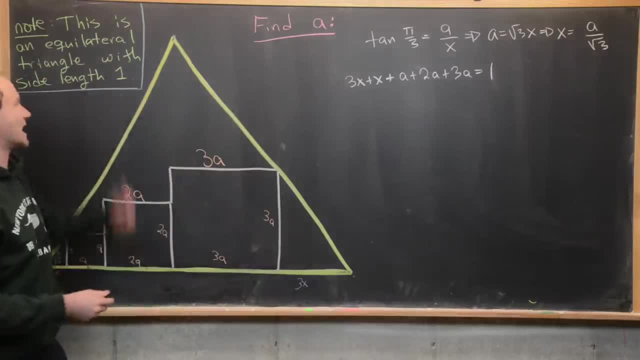 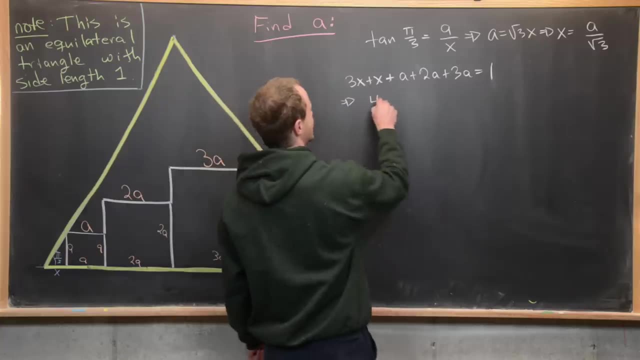 because that's comprising the entire side of this equilateral triangle with side length 1. but now notice, we can combine like terms here and we get 4x plus 6a equals 1. next we have a value of x in terms of a from this trigonometric relationship that we talked about. 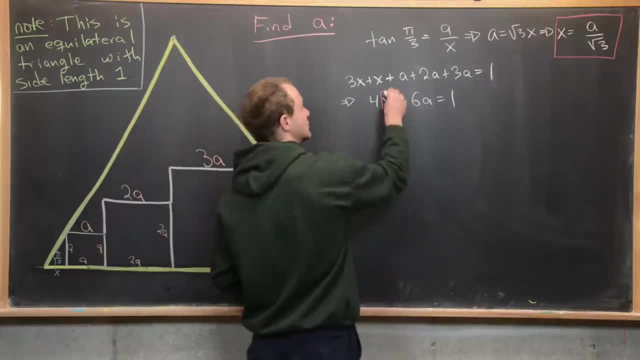 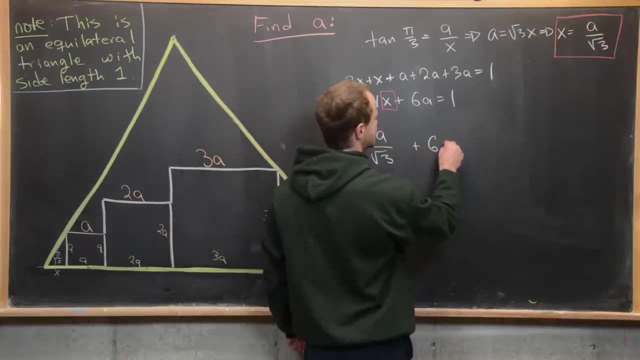 so we can input that into our equation down here. we're going to have 4a over the square root of 3, plus 6a equals 1. let's go ahead and rationalize the denominator here, so we can do that by multiplying this by the square root of 3 over the square root of 3. 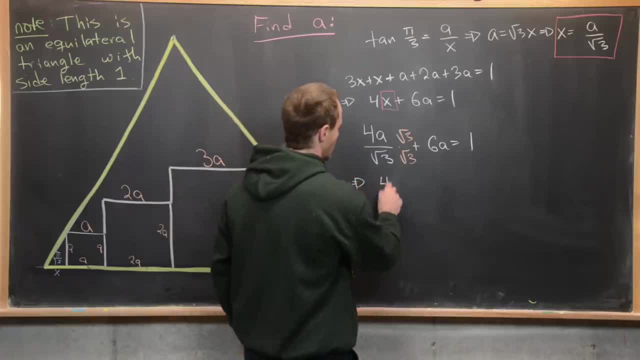 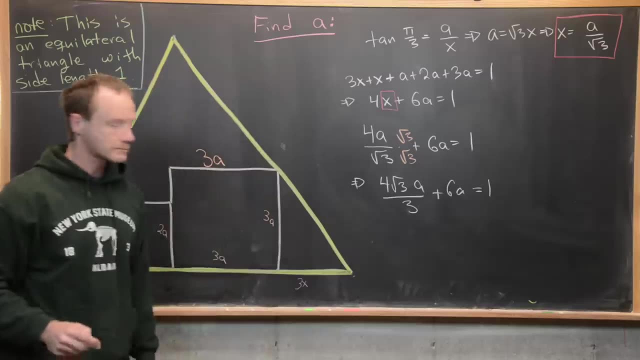 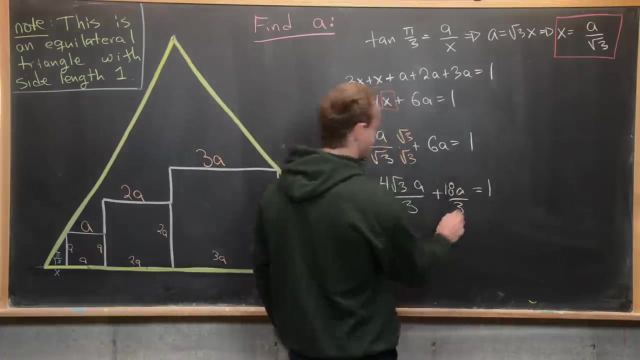 so that's going to give us 4 times the square root of 3a over 3, plus 6a equals 1, so let's maybe give this a common denominator of 3, so we can rewrite 6 as 18 over 3. 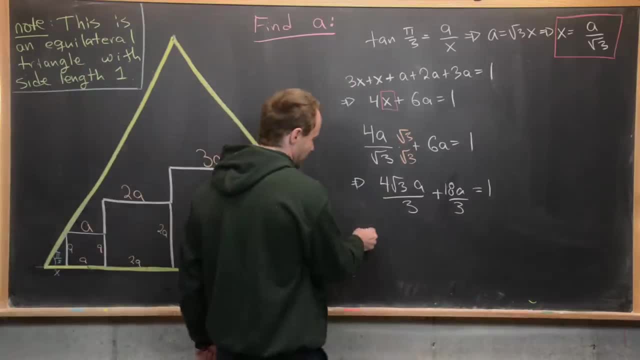 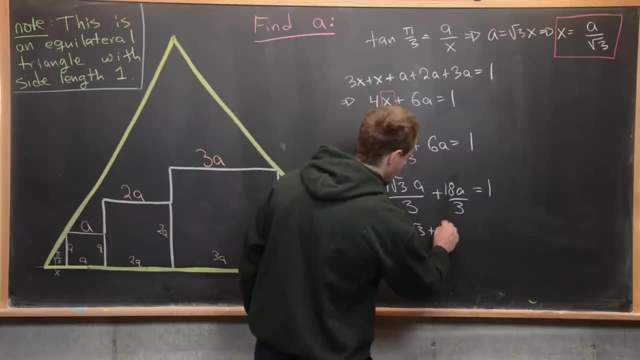 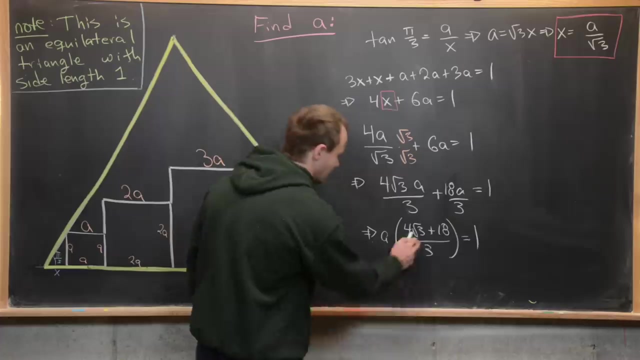 then next we can factor an a out of the left hand side. that's going to give us a times the quantity 4 root 3 plus 18 over 3 equals 1, great. so we can multiply by the reciprocal of this number and we get a. 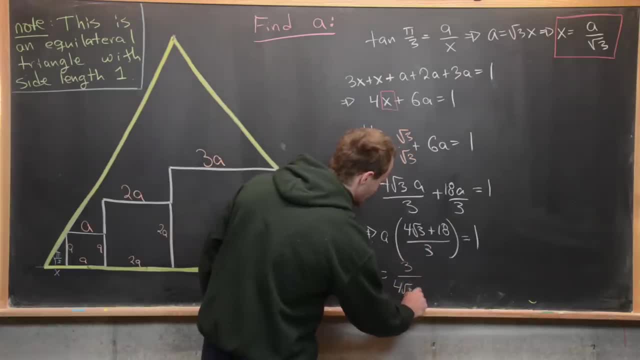 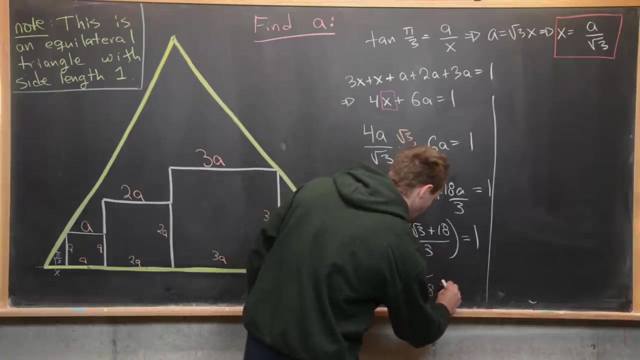 equals 3 over 4 times the square root of 3 plus 18. and then next, perhaps we'd want to rationalize the denominator, although in my mind that's not strictly necessary. but you could do that by multiplying this thing by 4 times root. 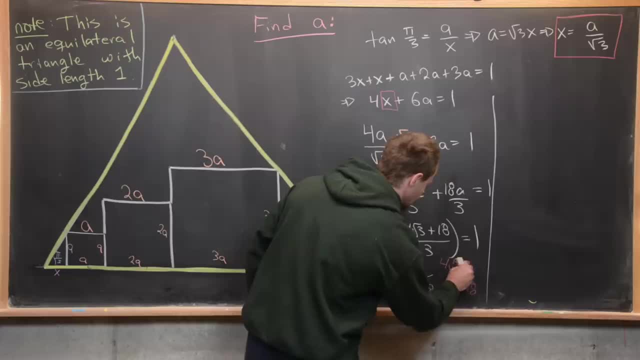 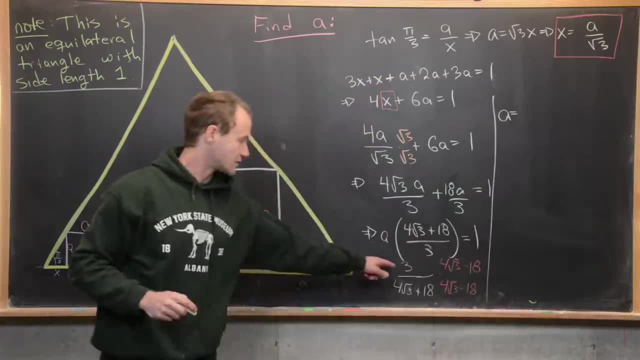 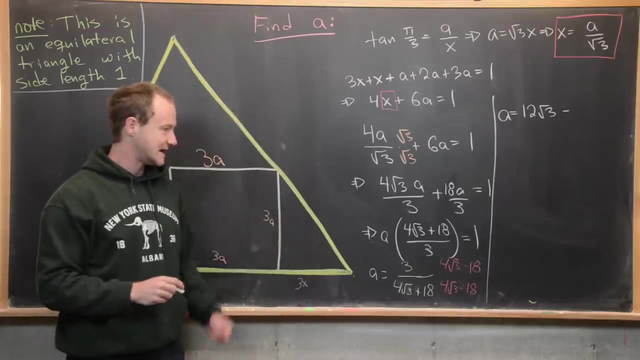 3 minus 18 and 4 times root 3 minus 18. so let's see what that gives us. that's going to finally give us a is equal to: so this is going to be 12 times root 3 minus 3 times 18. so let's see what that is. so 3 times 18 is going to be 54 over. 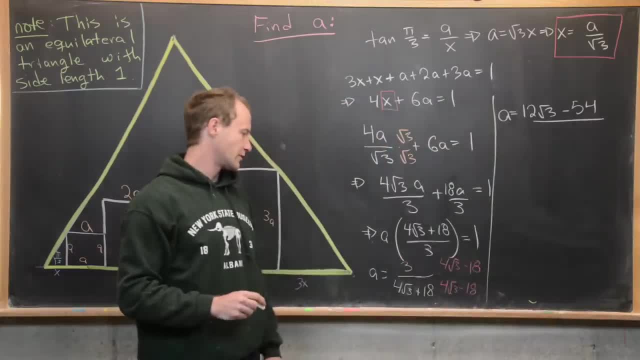 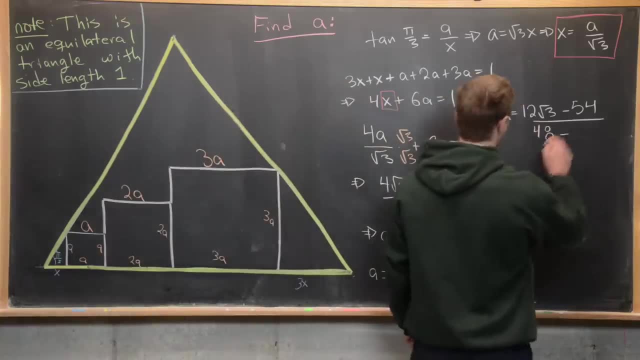 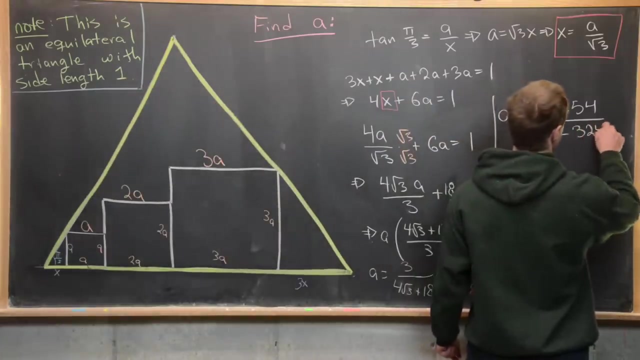 now we're going to have 4 root 3 times 4 root 3, so that's going to be 16 times 3. so 15 times 3 is 48 minus 18 squared, and 18 squared is 324, so 324. so next, maybe we'll simplify. 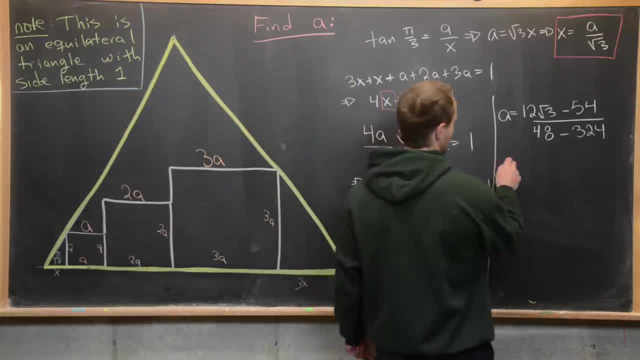 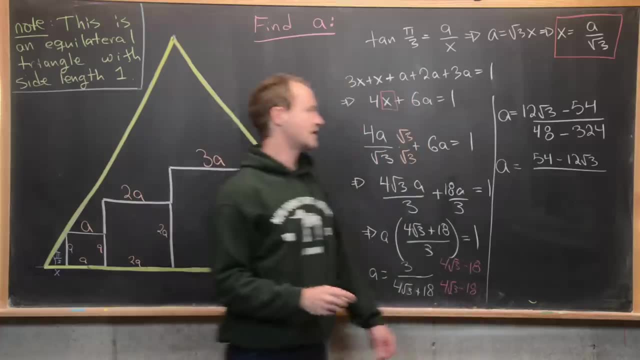 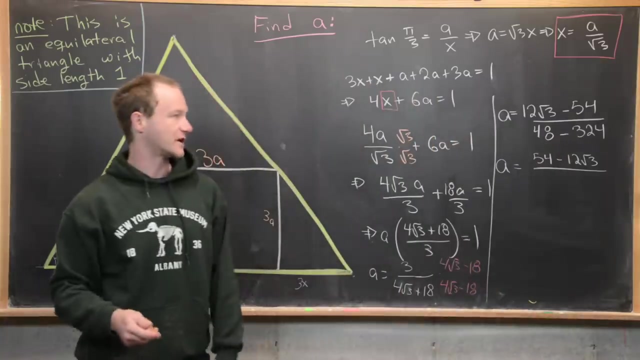 this by changing the order of the numerator in the denominator. so I'm gonna write this as a equals. so 54 minus 12 root 3 over, well, what's 324 minus 48? so that is going to be equal to. so minus 124 will get us down to.